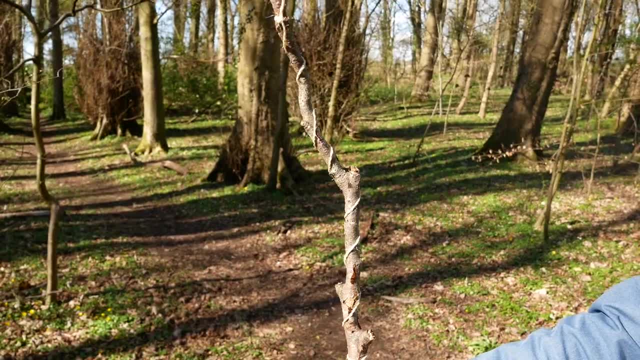 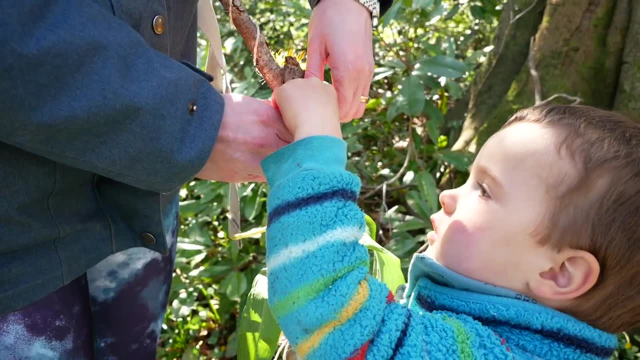 and you need to take some twine. You just tie it to the top, wind it down a little bit and then tie it around halfway down. The idea is, as they walk through the forest they can collect things that they find interesting and just tuck them into their journey stick Ben is so excited when he walks. 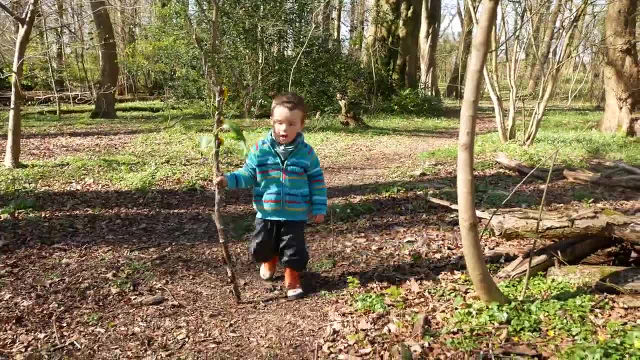 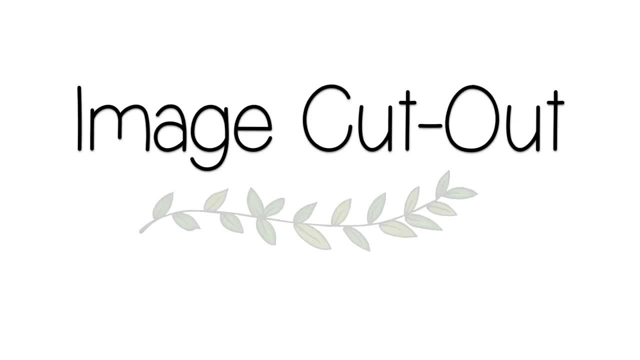 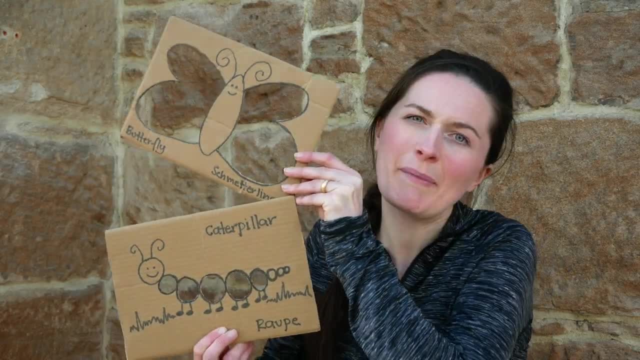 through the forest with one of these- and he is always so proud of what he creates- And then, obviously, make sure you take that twine away with you as well when you're leaving. My next activity is to create some cardboard cutouts. Now I just made these ones. I drew some pictures that made. 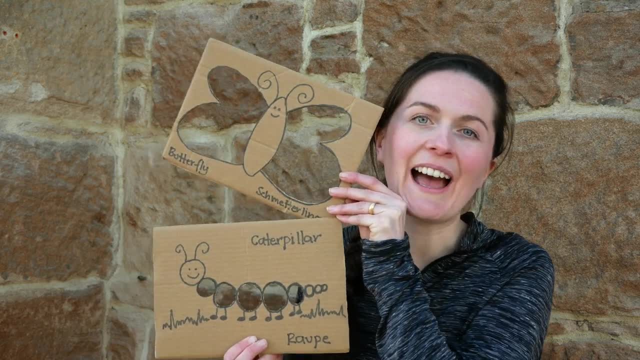 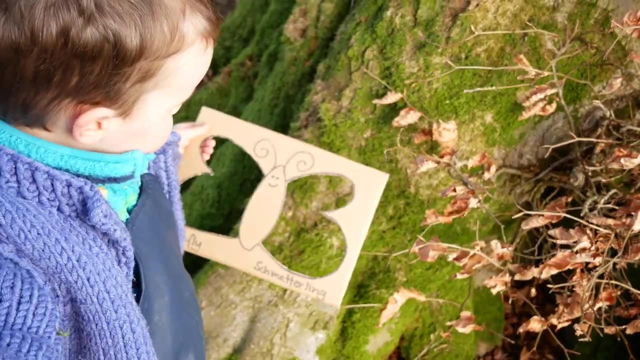 sense for when we were outdoors and then, using a craft knife, I just cut out the holes. Then, wherever you put them, you can see through them and see whatever background is there. so you can hold them in front of flowers, Either using a craft knife or a paper towel. you can see the background for each. 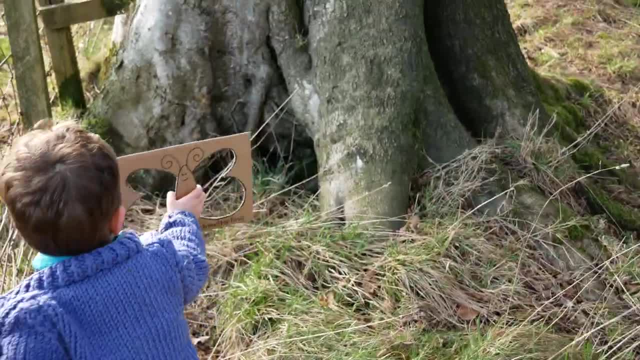 one of the boards If you want to keep them and use your own as a base for your in front of different plants, in front of bark, and they're always going to make, in this case, your butterfly or your caterpillar look different. Next, I would 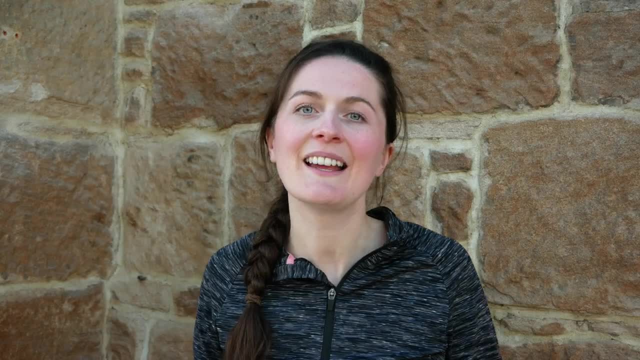 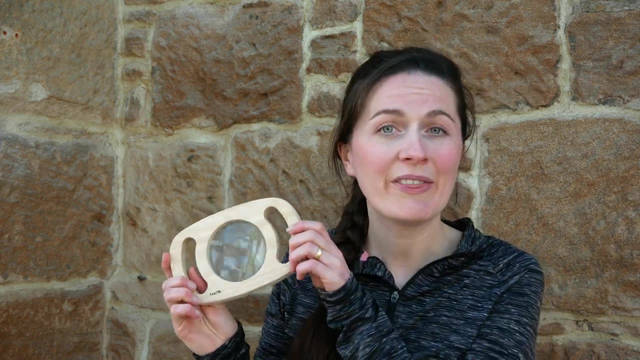 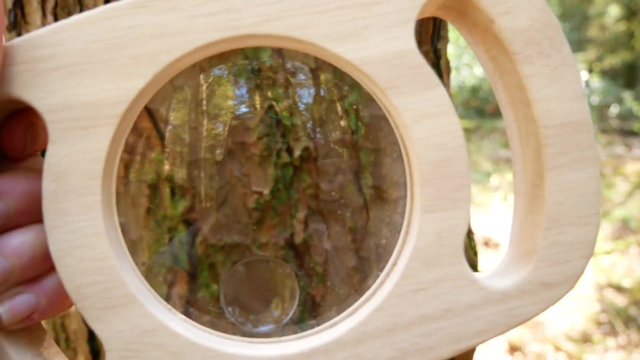 totally recommend getting hold of a magnifying glass. We recently picked up this one. it was actually Ben's Easter present and I will link it below because I would totally recommend it- With the two handles. it really helps toddlers to be able to position it and it's pretty light as well. Then, when you're out on a 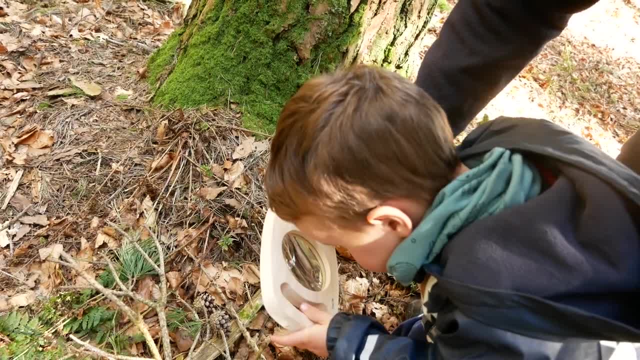 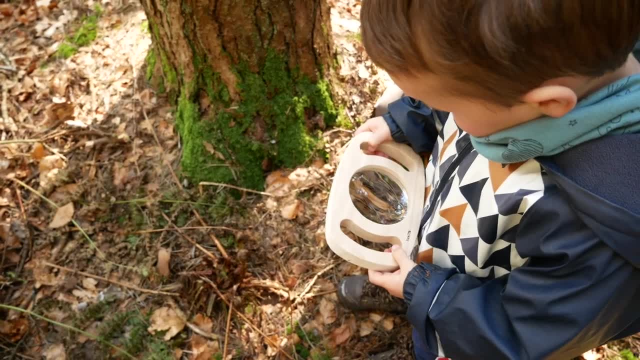 walk. you just take your magnifying glass with you and you can look at closer, at things like leaves, pangolins, bugs. There's so much to discover and it's really fascinating when you can actually, for example, look at all the tiny legs of. 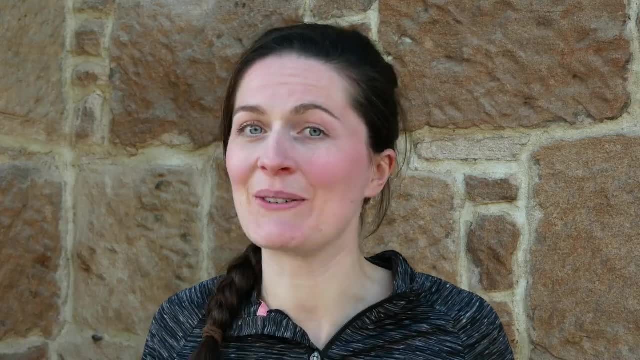 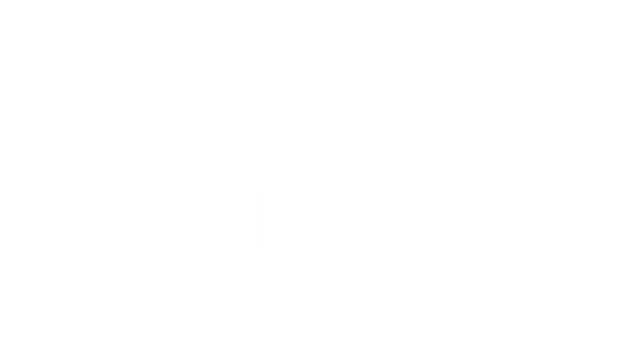 a millipede. I also think this is something that he's really going to grow into and use more in the years to come too. My next activity is definitely a classic, and that is to do some building in the forest. We have a few different. 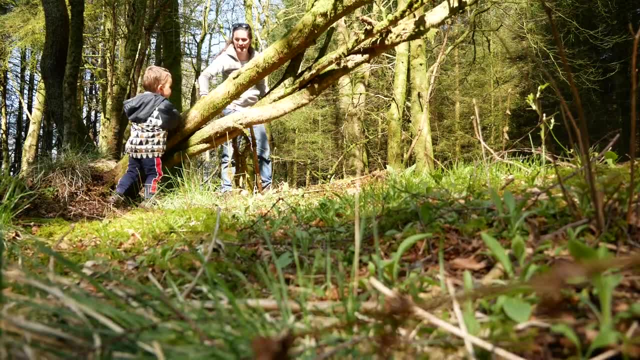 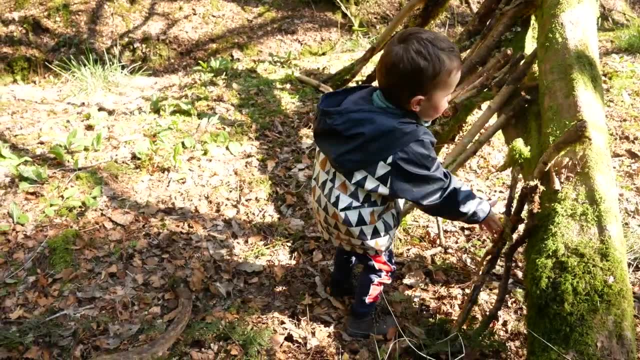 versions of this activity that we really like to do. The absolute classic is building a den, which is really easy with just finding a tree that's at a bit of an angle and lots of sticks. Ben also loves to add some extra touches, like building a little. 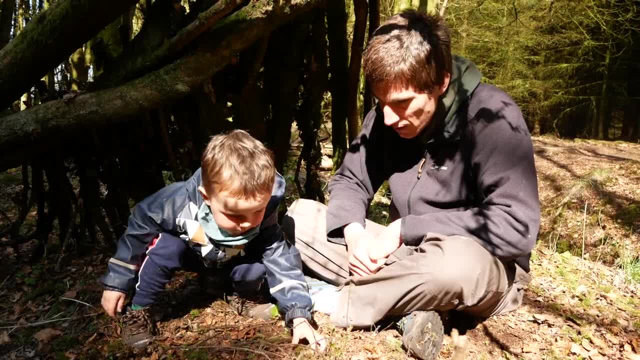 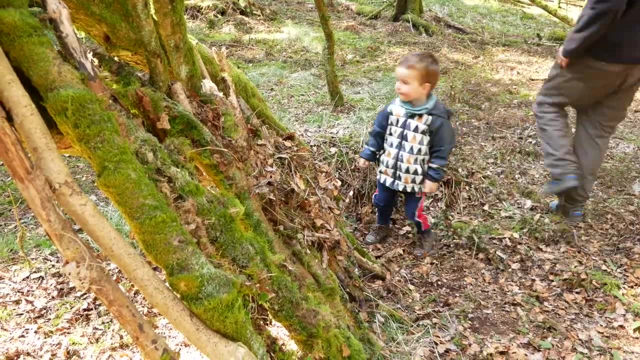 pretend campfire. This, I think, is also an activity that Thomas and I really enjoy doing most with Ben, and you can also take, for example, a tarp, if it's a bit wet, to sit on inside your den and have a little snack. Another version of this is to do: 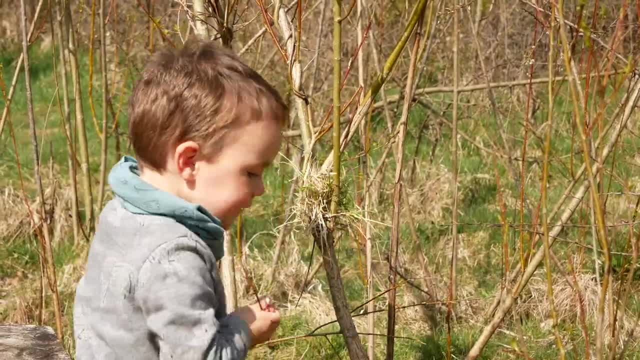 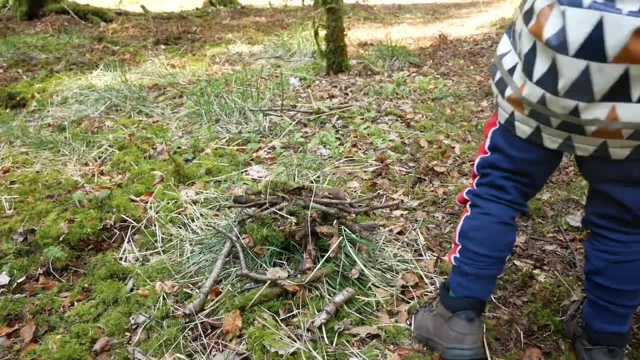 some bird hunting, The bird nest building. Ben is very into this at the moment because he is really loving birds. It's just collecting things like dried grass and leaves and sticks from around the forest floor and turning them into the shape of a little bird's nest. We 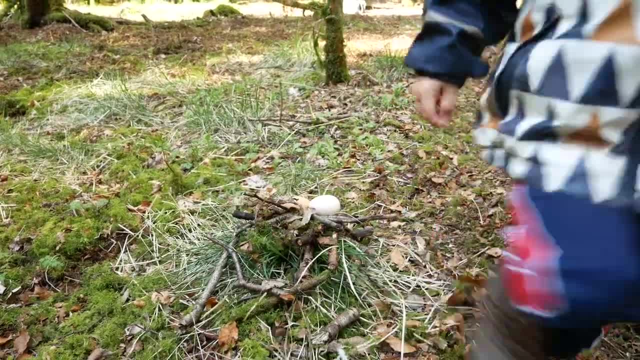 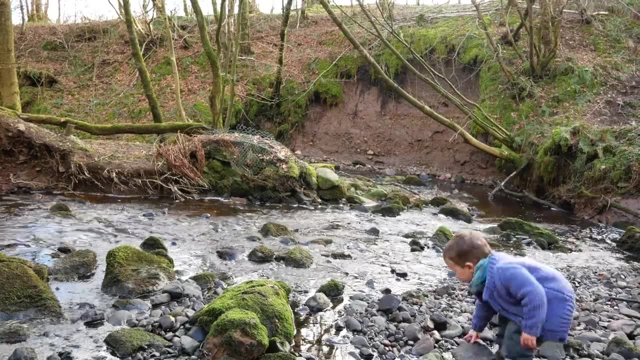 also take some of our sorting eggs, which Ben can then put on them, and he loves to pretend and talk about what type of bird nest it is- And the final version here is to do a little bit of dam building at a small stream. Now, obviously you have to be. 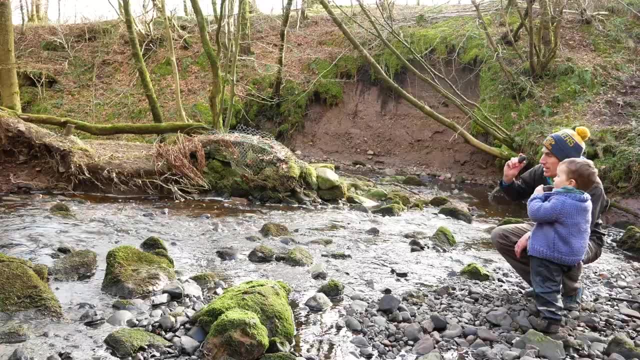 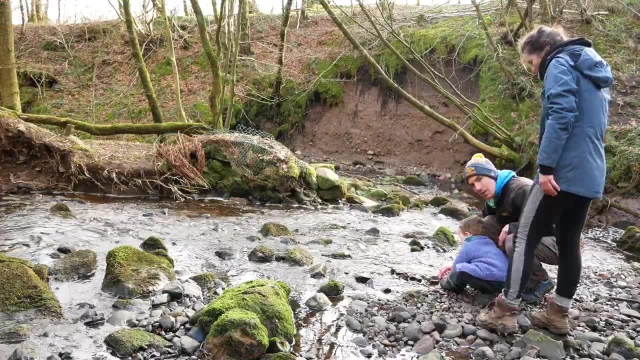 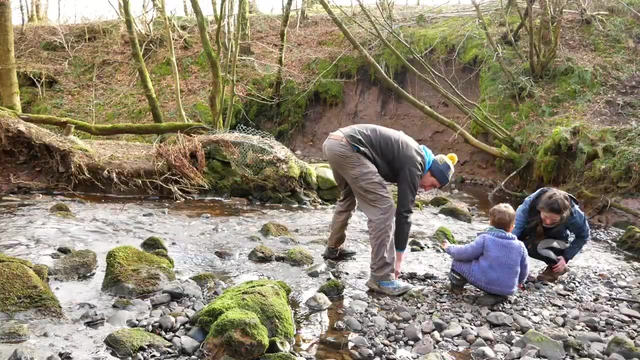 a little bit careful here that you're always supervising your child near water and it's not so deep that they may fall in and get wet and very uncomfortable. However, this is a really nice one for them to watch the flowing water change its course, perhaps just a little bit. Thomas, particularly, is a huge fan of 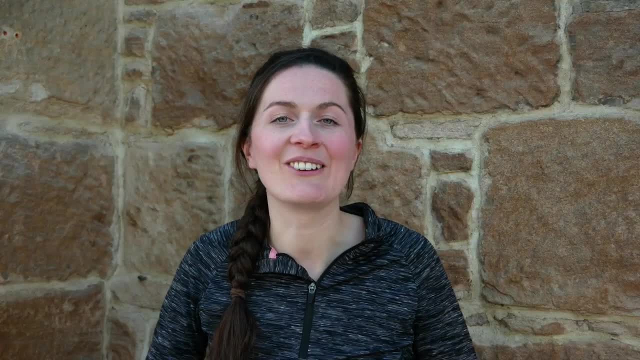 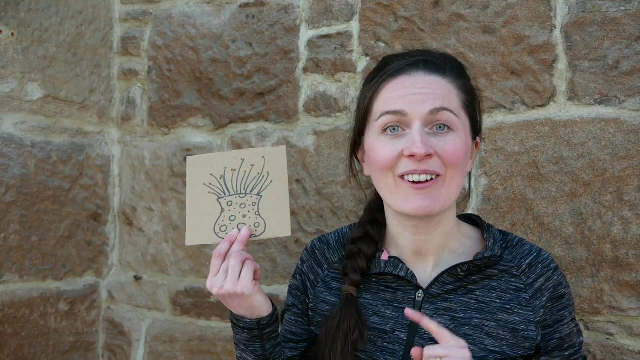 this one because he has a Geography degree and loves sharing some of that knowledge with Ben. My next activity is to create a cardboard vase. So to make this, I just took a piece of cardboard from a recycling, drew a little vase on it, some stocks. 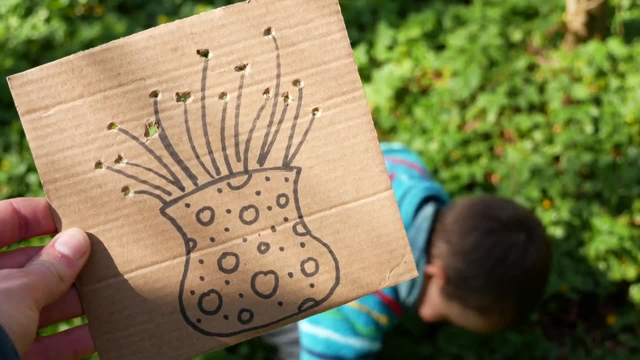 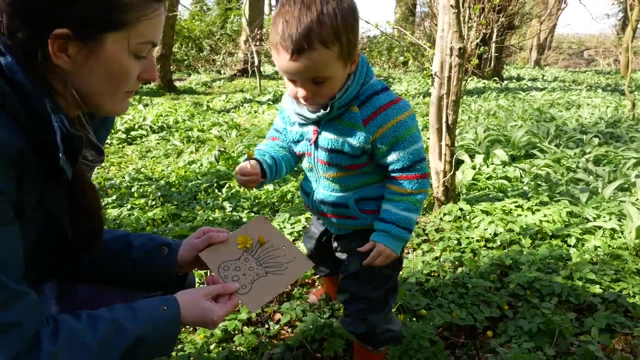 and then poked some little holes through it just using a toothpick. The idea is that you can pick flowers and then thread them through and it looks like a full vase of flowers. Now I would totally recommend caution with this one. We try to encourage Ben not to just pick flowers, because 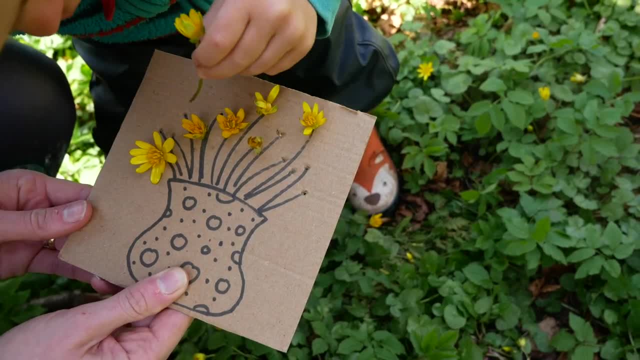 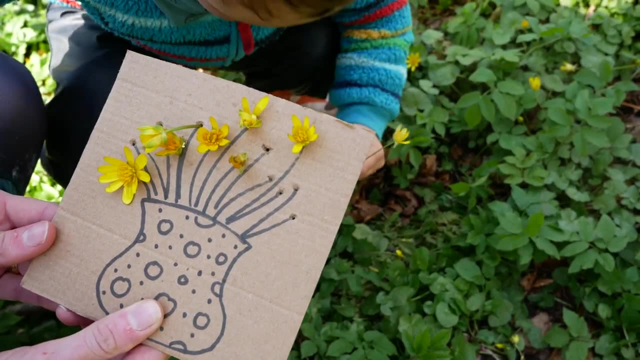 obviously they're there for the bees and for other people to enjoy. I only ever do it if the flowers are going to be used for another purpose or if, for example, the grass is about to be cut and the heads of the daisies and buttercups are going to be chopped off. So that's a really good idea to do. 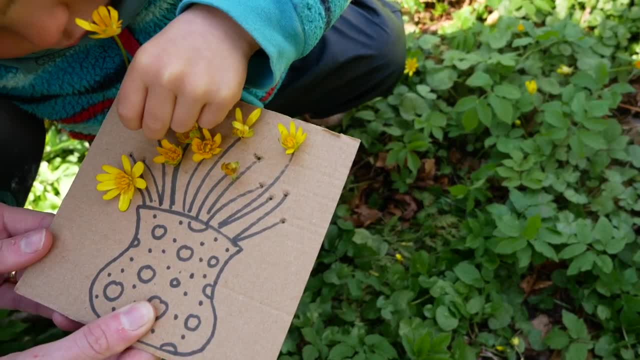 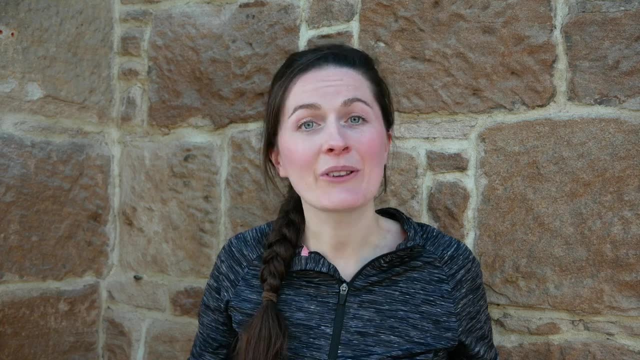 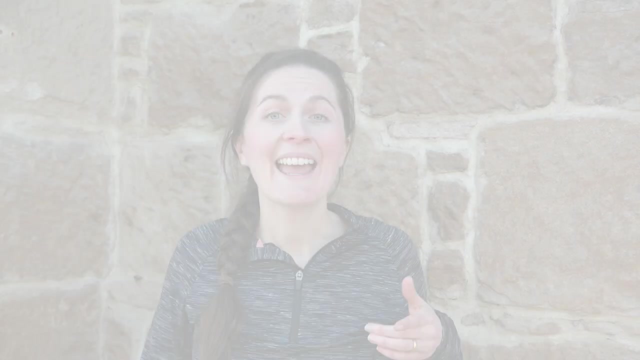 With the ones that Ben picked for this. they're later celandines, a type of buttercup, and we're actually making some wildflower artwork. We're pressing flowers, so they're going to be used for another purpose too. My next activity is nature cutting, which definitely follows on from that. 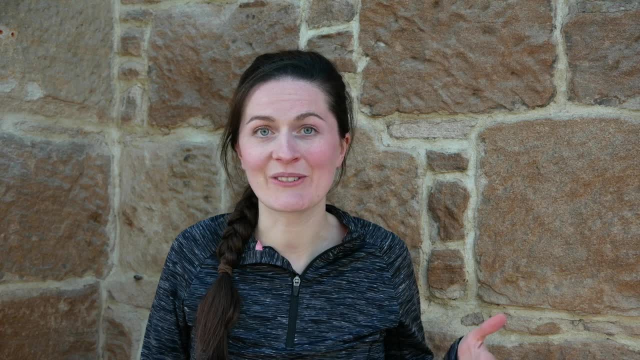 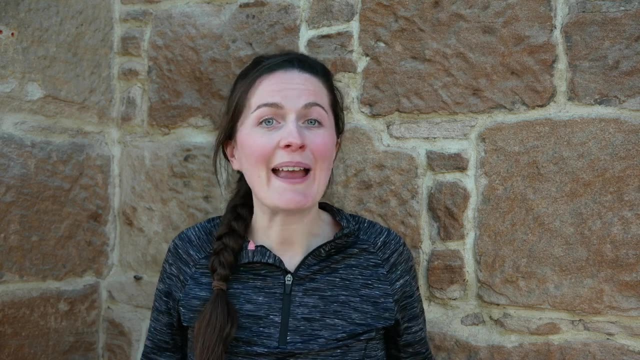 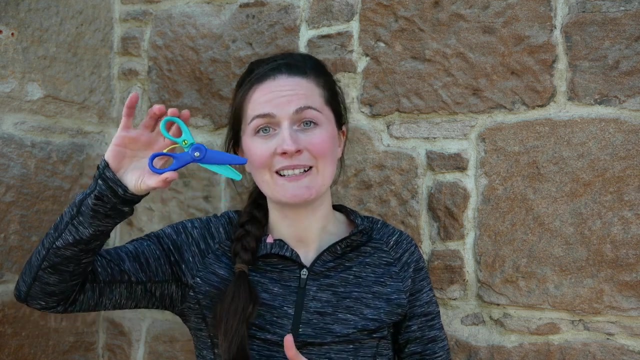 Anyone. I said that we only cut or pick things that are going to be used for another purpose. We are big fans of foraging, and right now is a great time for wild garlic, So Ben took his scissors to the forest. These are fantastic. I have talked about them before, but they're so good because when Ben 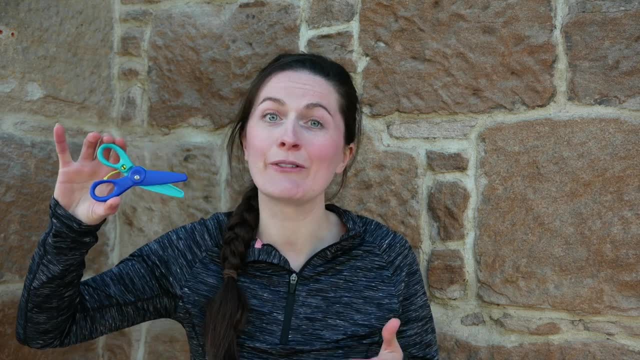 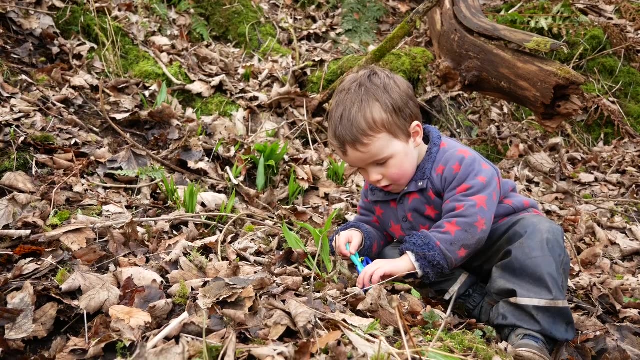 presses closed, then they just ping back open, So it's a really great way for toddlers to learn to cut. I'll link those below as well, But we take these with us and Ben can cut the stalks of the wild garlic and collect them in our bag. I think that foraging is a great way to connect toddlers. 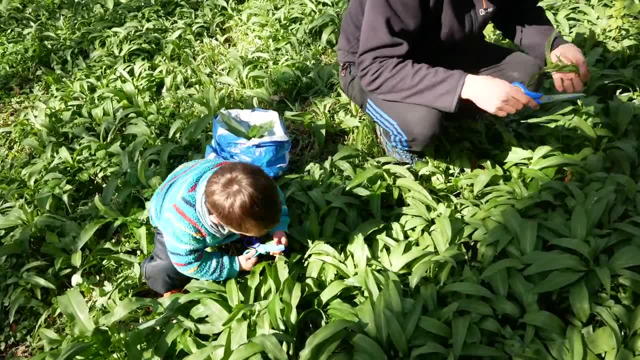 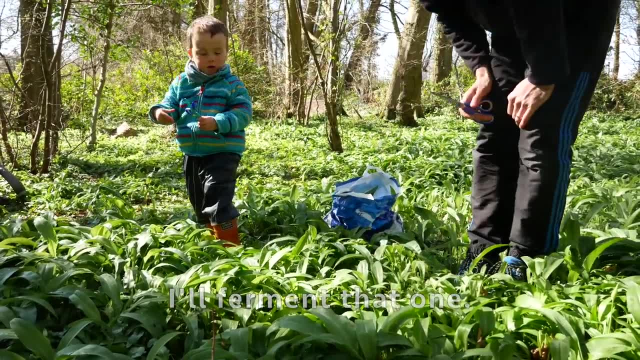 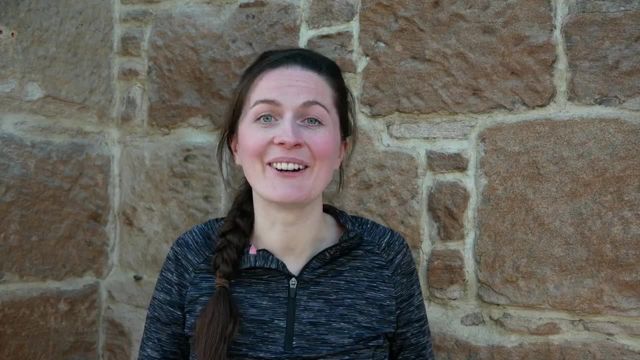 with nature, and I also think it's so important for them to learn what things they can eat and what things that they certainly can't Give the bug to you. I'll remain that one, Okay, Super. If, however, you're not at all comfortable with the idea of foraging, you can also do this just with 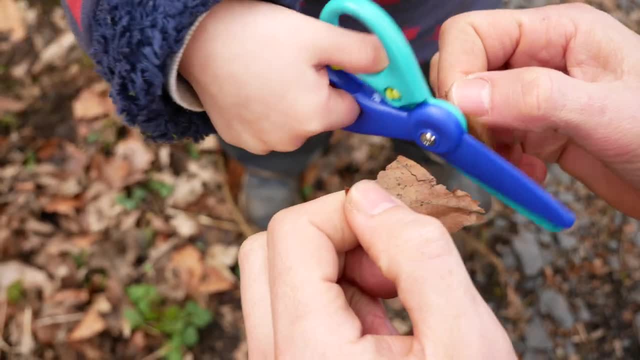 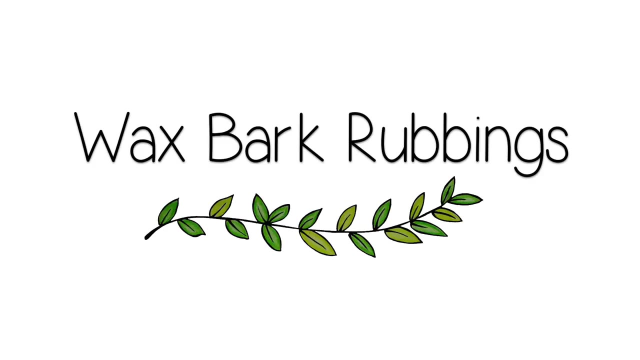 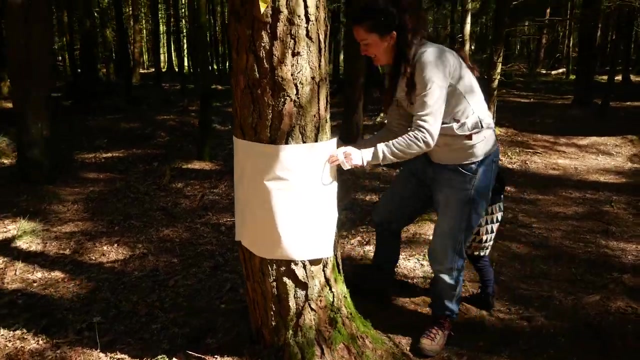 leaves that you find on the ground. It's really nice, for example, to cut it up into lots of little pieces to make leaf confetti for a post-covid celebration. Activity number seven- another classic- and that is to do some bark rubbing. So really simply, you can just take either sheet of paper or 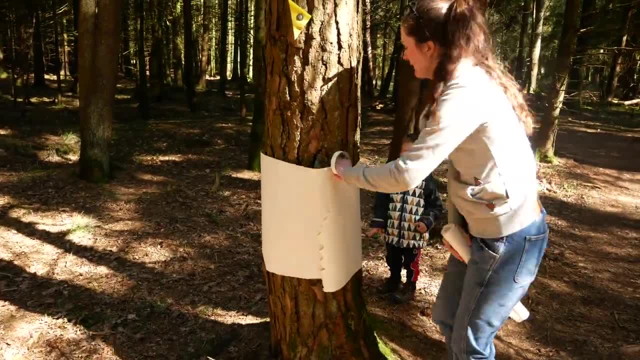 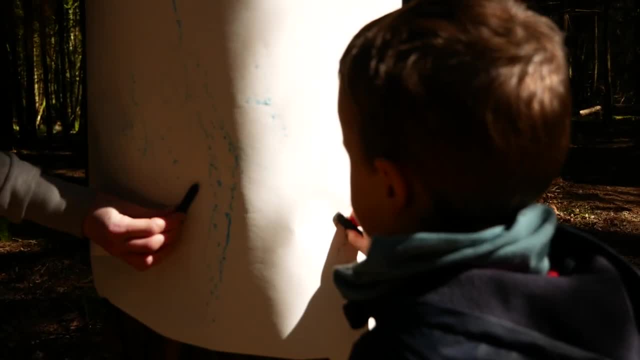 we absolutely love to do some bark rubbing. You can just take either sheet of paper or we absolutely love these big Ikea rolls of paper and tape them to a tree or around a tree. just using some masking tape tends to work pretty well. Then, using a crayon, you can take rubbings of the bark. You can also 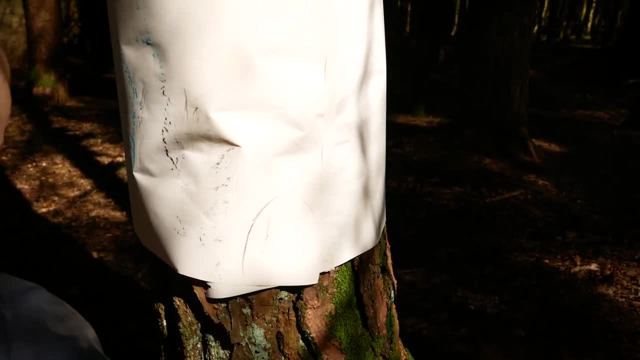 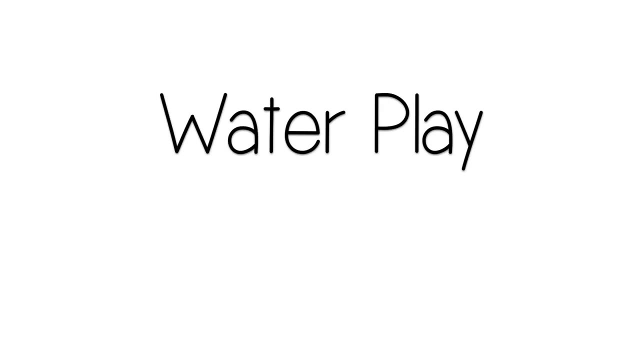 just collect some leaves when you're out and about and do this with some leaves at home. It makes some really beautiful pictures that then, for example, I like to cut out and put on cards. My final one is definitely the easiest and the one that is definitely Ben's favourite, and that is to find a 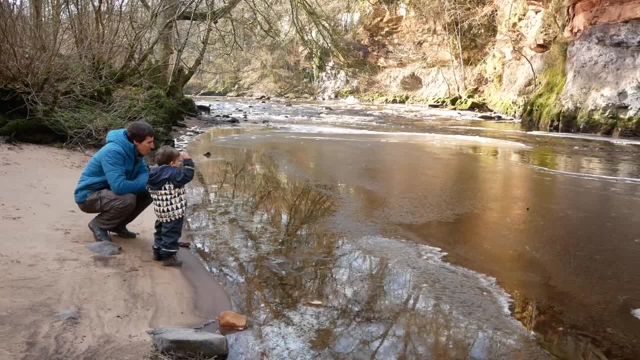 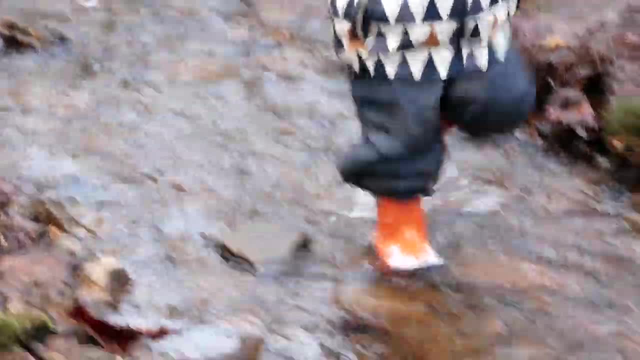 little shallow stream or bog. It's a big puddle to do some water play. So nearby where we live we have a forest which has a very shallow little. we call it Ben's mini gorge walk. He can just walk up and down as he pleases, splashing in it, throwing. 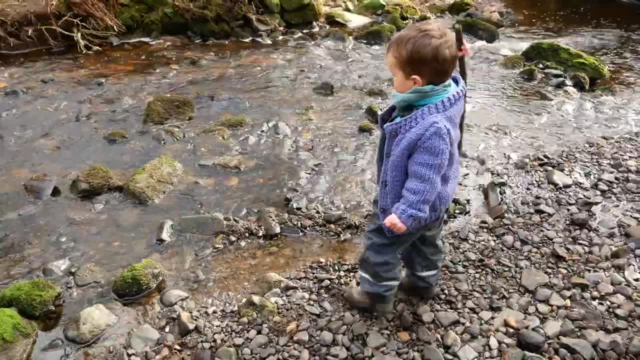 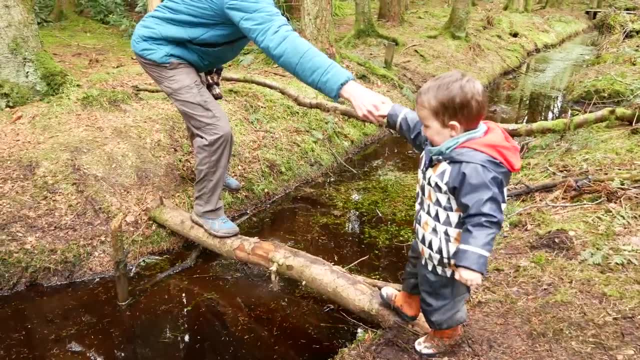 stones in it, sticking sticks in it. The play potential here is endless and Ben would spend the whole day just playing in this little stream. And if you don't have easy access to one, a paddling pool with a shallow bit of water, some wellies and a little bit of water will do the trick. So if you don't have easy access to one, a paddling pool with a shallow bit of water,